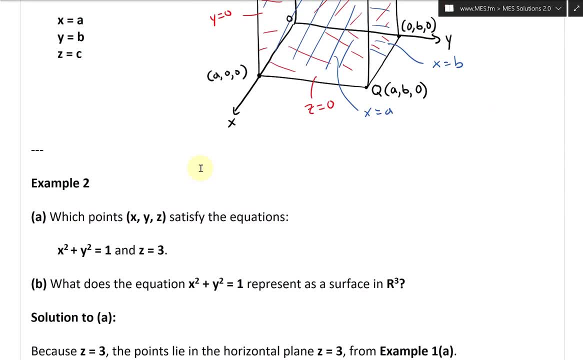 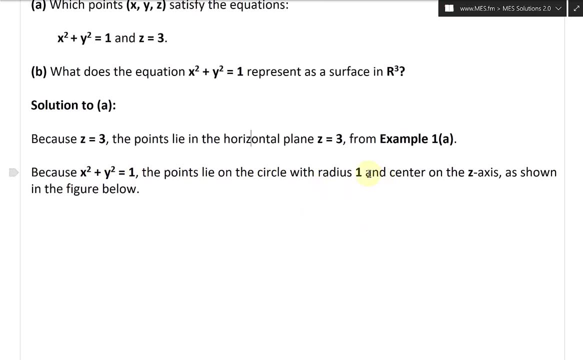 going to be somewhere along this there. But then we're also given an equation of a circle. This is just an equation of a circle, So because x squared plus y squared equals one, the points lie in the circle with radius one and the center on the z-axis, as shown in the figure. 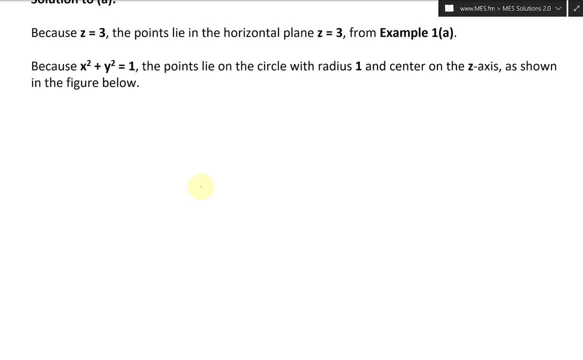 below. So we draw this out, We're going to have something that looks like this: This is our z, And there's our y-axis, our x-axis, There's the origin And this is our point three. And now we have it like: 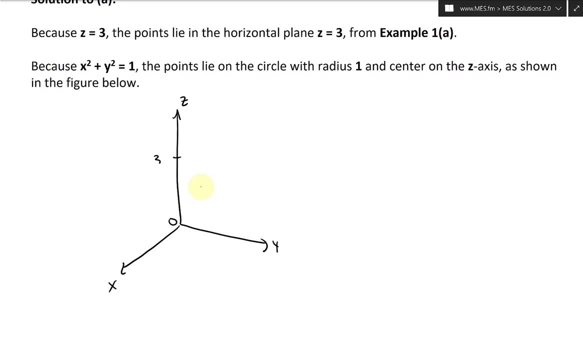 that I'll make it a bit shorter. Then we have a point three here, And now we're now. so that's a three on the z. But now we have x squared plus y squared, That's the circle. on this, z equals three. 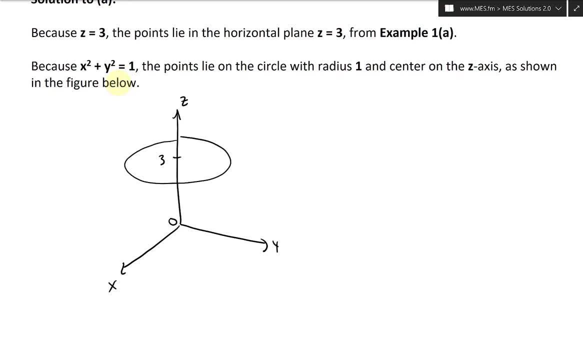 line. So we can write it like this, Draw it like this. So there's a circle And yeah, that's just our circle there And well, it's going to be behind this. So let's make this like this: dash. 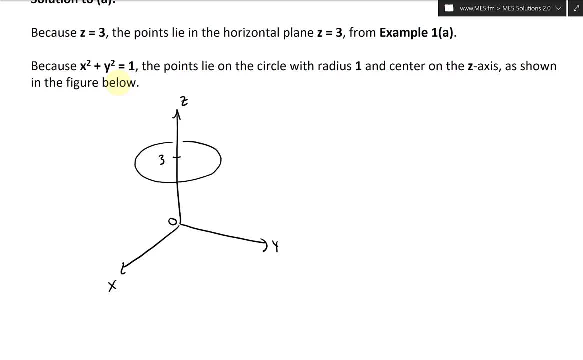 Let's try this one more time. All right? Yeah, So just have it like that. So this is going to be our circle? Yeah, So it's going to be circle. And the equations are: circle: x squared plus y squared equals to one And z is equal to three. All right, So now let's take a look at the. 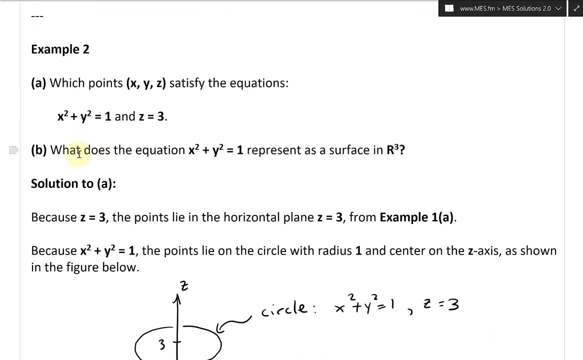 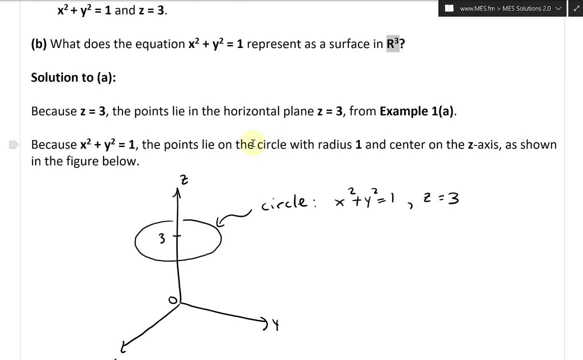 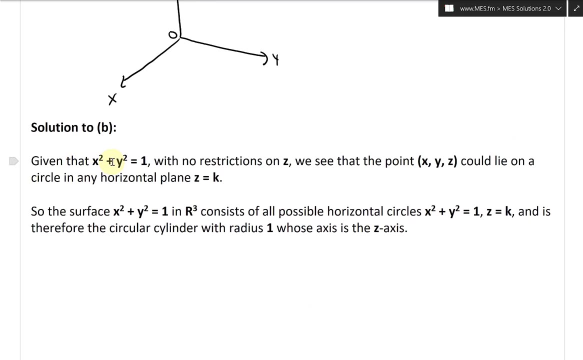 solution to b. So b is here. So we're given: what does the equation x squared plus y squared equals one represent as a surface in R3, in other words in three dimensions? And this is the same thing as this. but there's no z equals three. So let's take a look at the solution to b. So, given that, 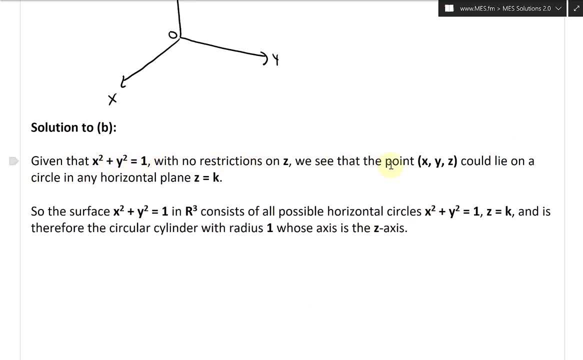 x squared plus y squared equals one, with no restrictions. on z. we see that the point x, z could lie on a, on a circle in any horizontal plane. z equals to k. So the surface x squared plus y squared equals one. in R3 consists of all possible horizontal circles: x squared plus y. 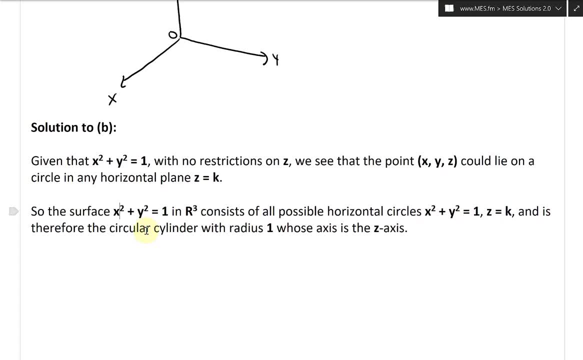 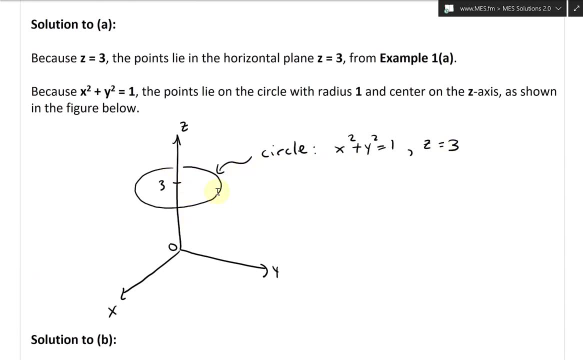 squared equals one and z equals k And is therefore: is therefore the circular cylinder with radius one, whose whose axis is the z axis. So basically, we're not limited to the z equals three. it could be on anywhere across. I'm just going to copy and paste that same graph here.